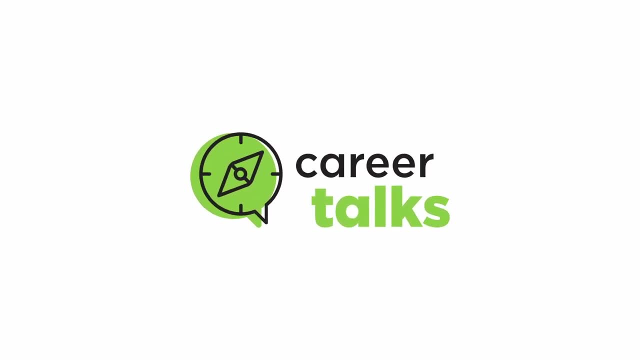 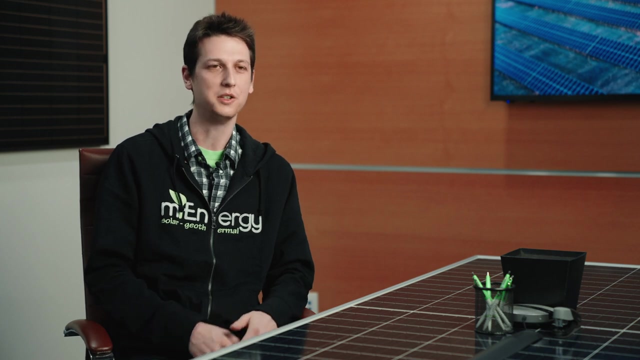 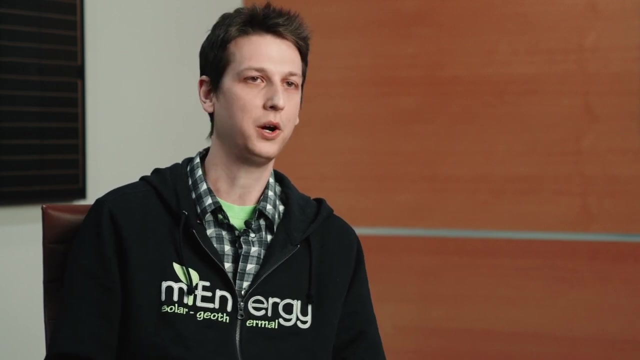 My name is Ryan Bogeen. I work at a company called My Energy here in Saskatoon. We specialize in renewable energy, so solar and geothermal. Our local company has been here in business for about 20 years now. I'm a project coordinator, so I do design, purchasing, project management. 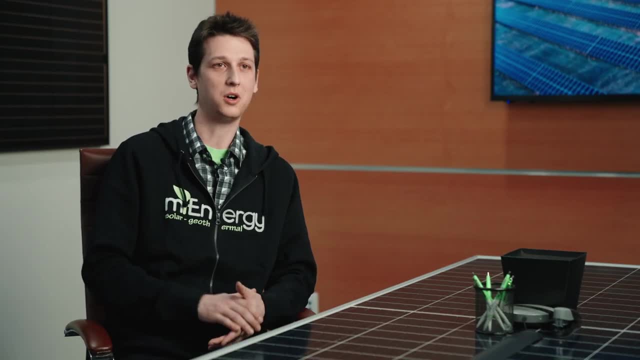 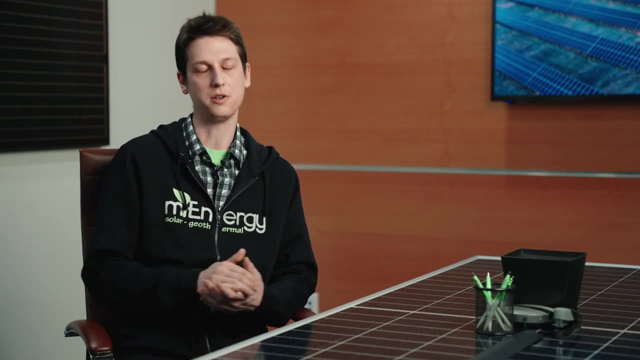 I mean, I wear quite a few hats, but I started as an installer very at the bottom, didn't know anything, and worked my way up where I was hands-on tools in the field, doing installs on your house, on your farm or whatever. 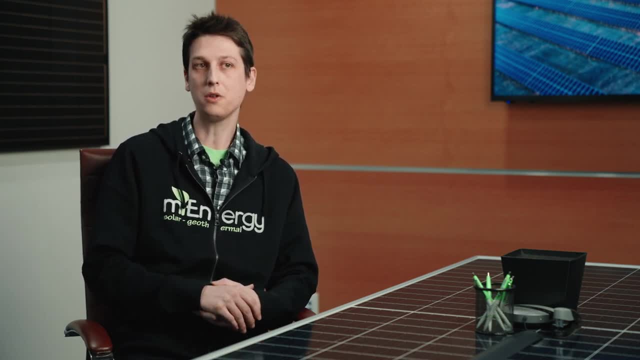 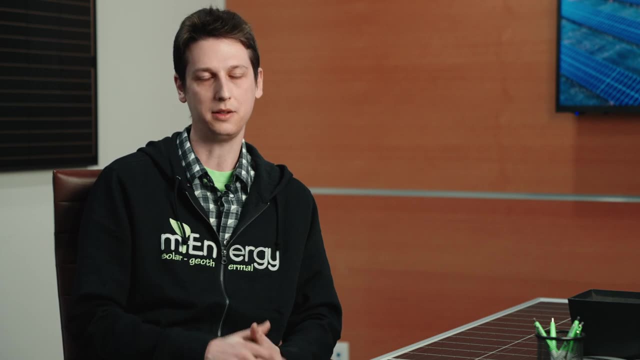 Shortly after that I was like: okay, now you're adding on purchasing duties, You've got to order the equipment. You know what you need. Now you've got to order it. And then soon after that it was okay. well, now I'm moving up to design as well. So not only can I get the stuff, but design it and go install it. 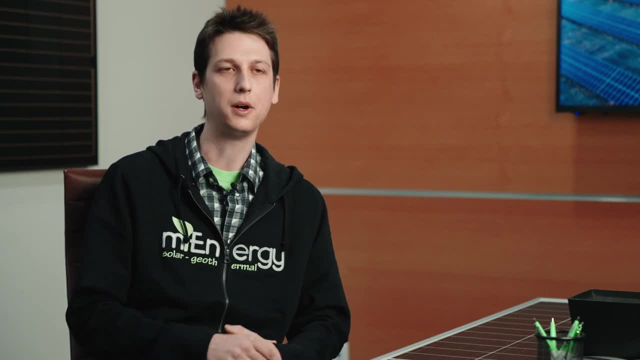 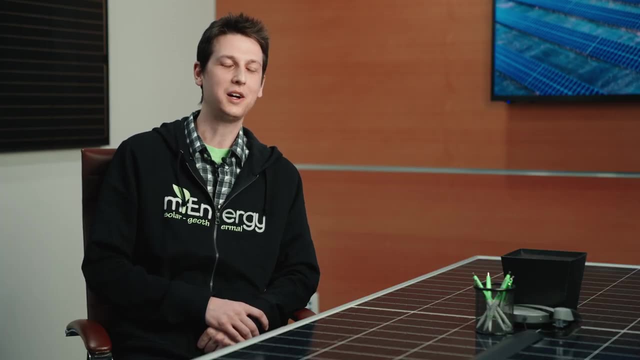 So I kind of did all those things for a number of years. Now I'm primarily focused on ordering And engineering where the company's grown enough. So yeah, in this industry, like my background and my education was in traditional environmental sciences- 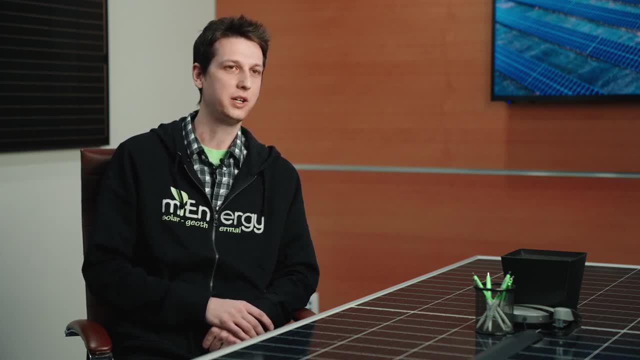 So it was in Alberta at a Lakeland College in Vermilion and it was testing soil science, water science, air science, that sort of thing where it was really kind of focused on oil and gas. I did that for a few years but didn't quite like the travel lifestyle and kind of bouncing from one place to another. 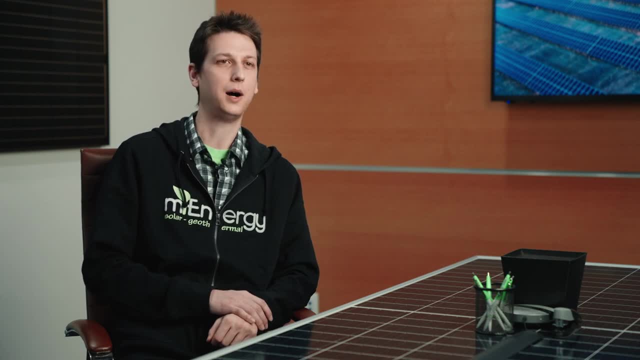 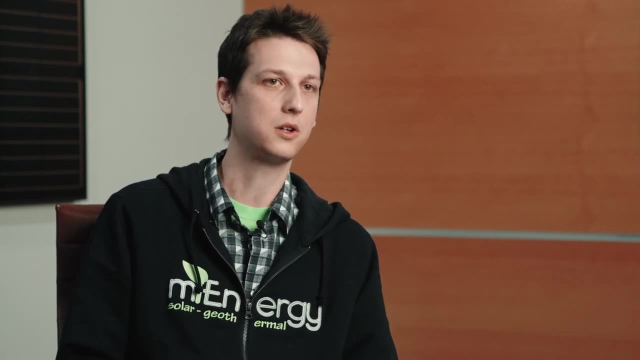 You've got to see a lot of stuff and it was really cool kind of exploring. But I wanted something a little more grounded and I found this here in Saskatoon where they were looking for a local junior-level installer for solar and geothermal systems. 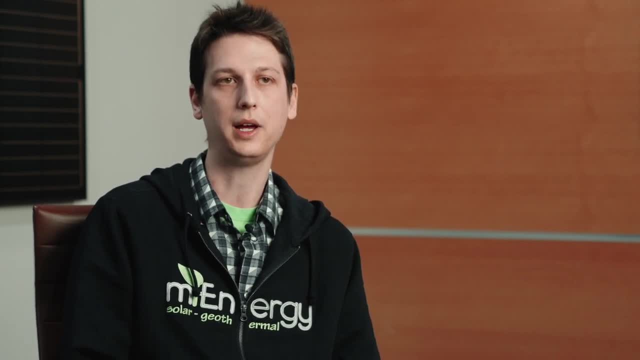 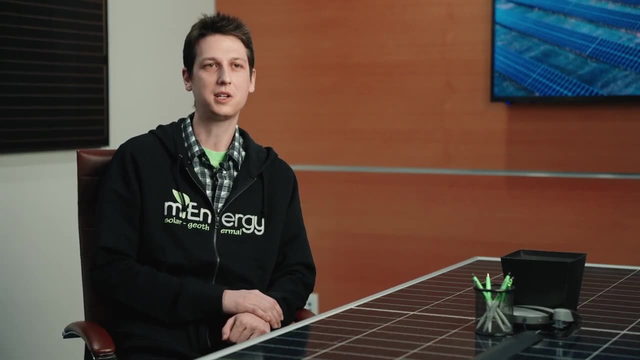 And I had done a project actually in college that was related to that, where I did a renewable energy kind of presentation for the class, And I just noticed that, hey, I know something about this, Let me apply. So that's kind of how I got my foot in the door was. I just said, hey, I know a little bit about it, I'm interested in it. 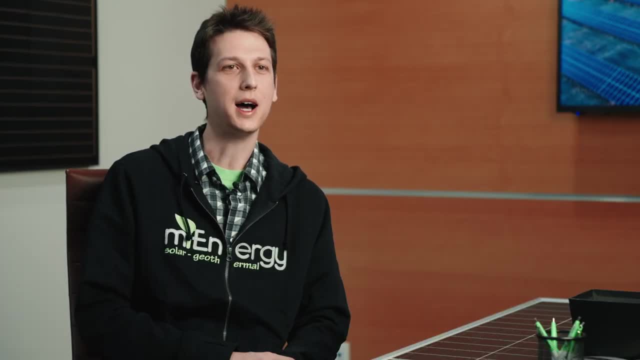 And when I was moving back to Saskatoon, that's where I landed. Yeah, I started Actually at university level, was getting my degree in- actually I think it was biochemistry. It shows that it was my first year. 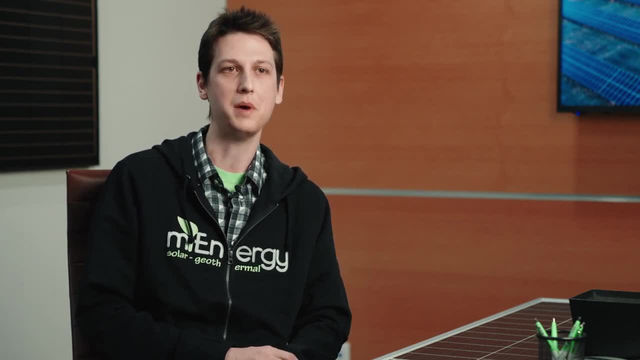 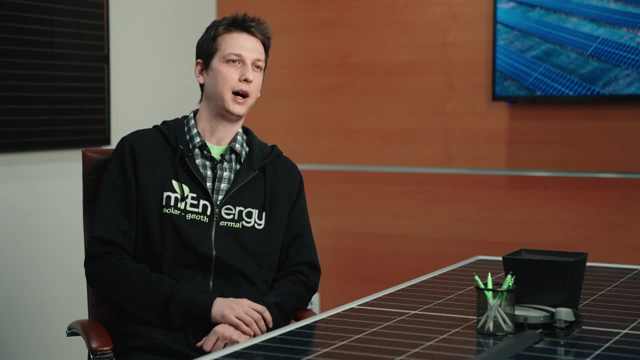 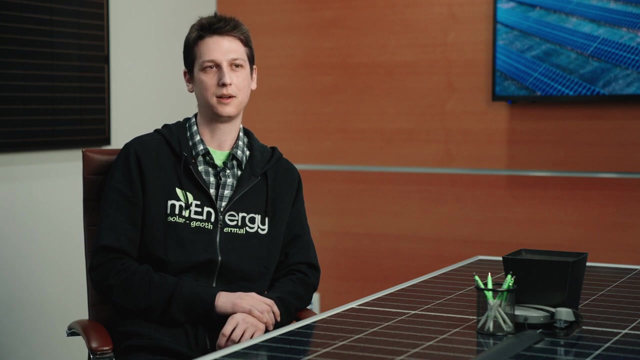 I was interested in sciences all throughout high school. Those were my best subjects, where I found those to be the most interesting and they came the most naturally to. me Did my first year at university and I pivoted over to college when I found that the class sizes and the hands-on wasn't quite great for my learning style. 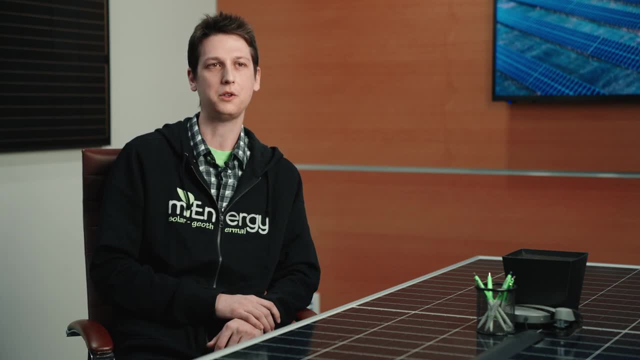 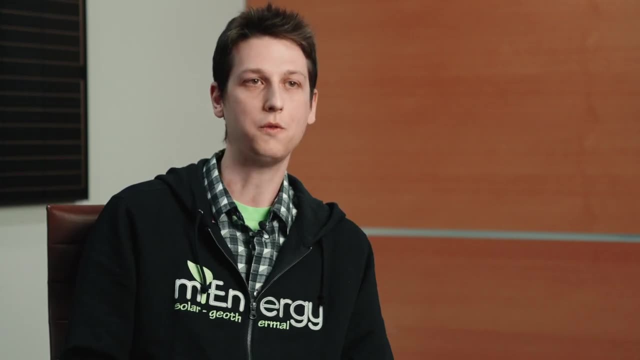 I was able to do it and be successful, but I didn't feel like I was retaining. So when I switched over to college, the class sizes were a lot smaller. There's typically less than 10 of us. You're out in the field, hands-on learning a bunch of different methods and different styles all at the same time, which I found very helpful. 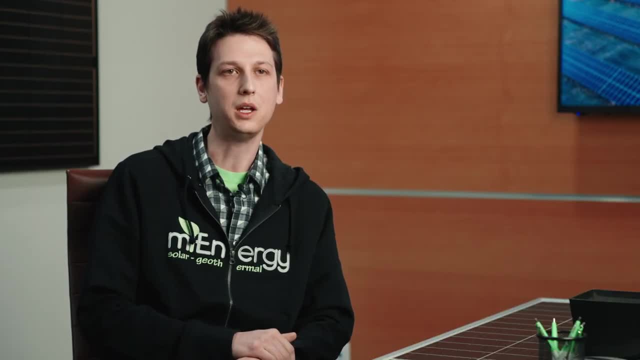 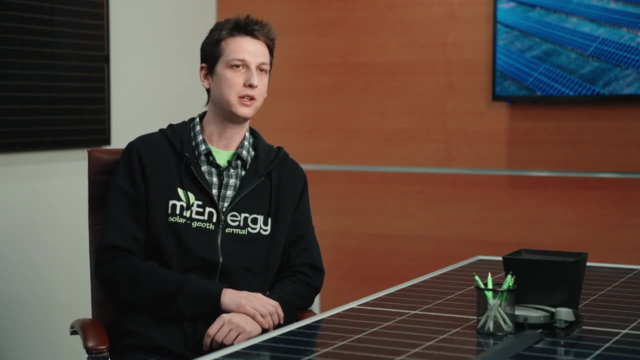 So that's kind of what I think was a better fit for me trying to develop a better knowledge base in science. So I have a Bachelor's of Applied Science in Environmental Management. It's a three-year program that has the last four years- three years of school. 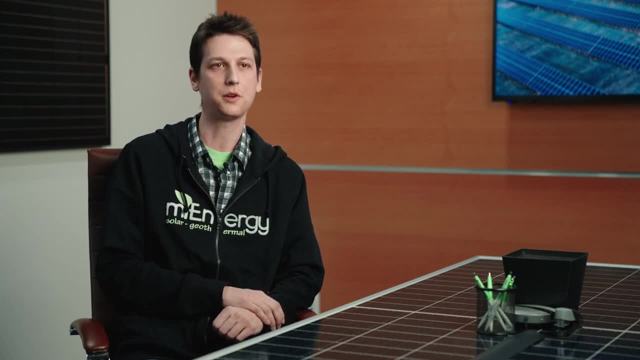 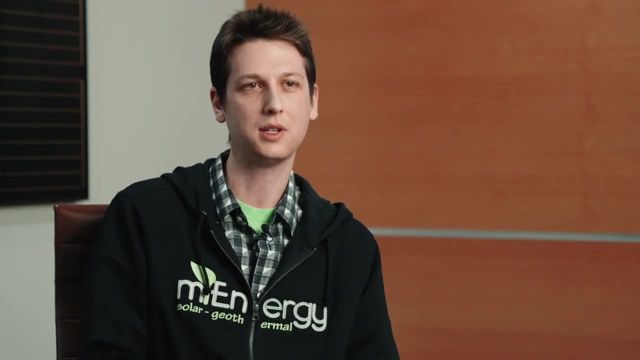 One year of basically work placement or practicum. So I actually got in my final year to go work in an environmental consulting company and do what I was trained to do because of my experience and being hands-on, and the teachers were like one-to-one. 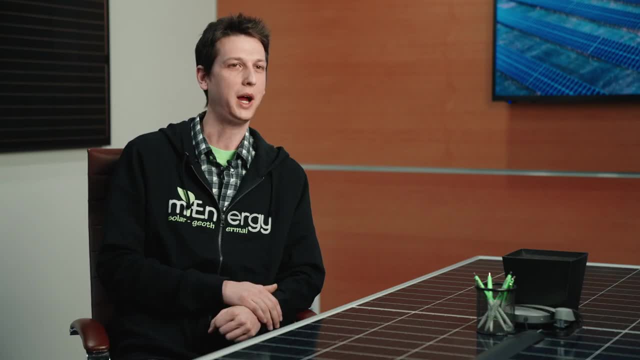 And it was really good. that way I was more prepared for the workforce. I wasn't kind of straight out of never doing any of this before and kind of fearful of what I might do. I kind of knew how to do a lot of this stuff. 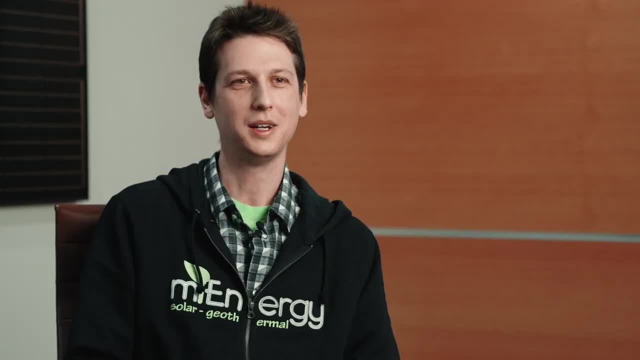 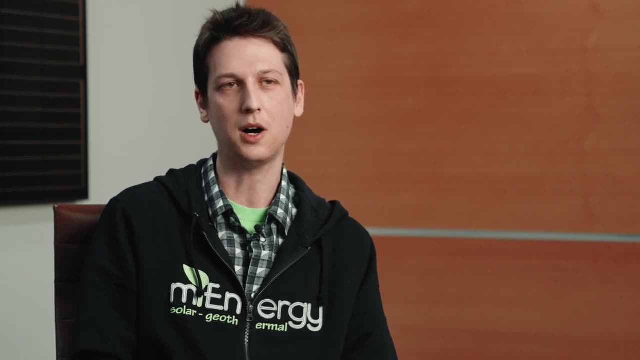 So that did really help me Get that position, get the job, and say, hey, I've done this before. Yeah, typical days are pretty diverse, where I've got a lot of stuff, a lot of juggling, where when you do wear many hats or do a lot of different roles in a company, when you've been here a while, it can get or seem kind of frantic. 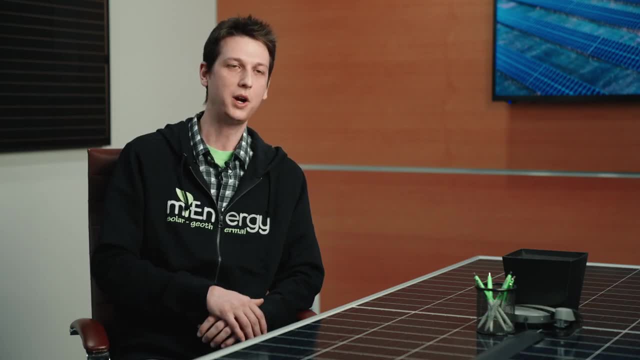 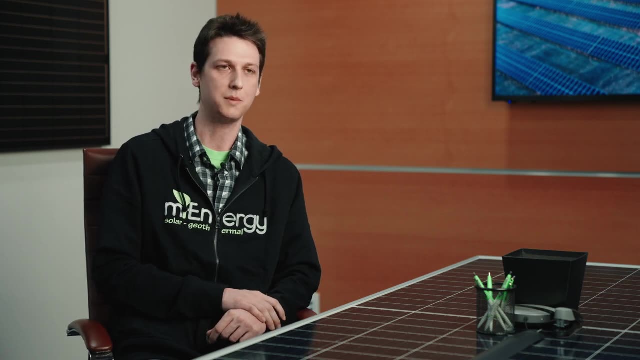 But planning for future jobs, handling past and present jobs with service calls or many different facets of planning, is typically what takes up a lot of my time, And also helping folks out where I've been here long enough, So I'm kind of a busy guy. 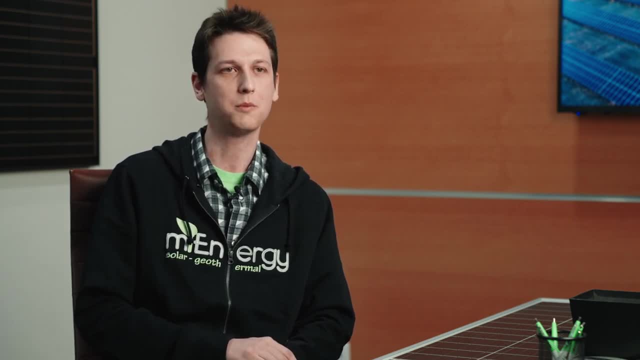 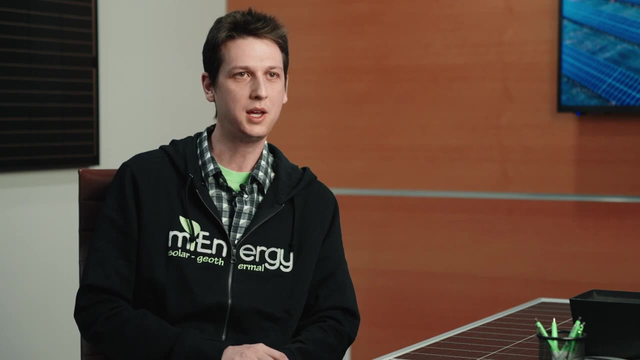 I'm kind of a bit of a resource where I can help folks out, I can kind of get them unstuck, I can provide some of my knowledge to, say, solve problems or whatever. So most of my day is quite busy, Feels like there's not enough hours in the day, but you get a lot done. 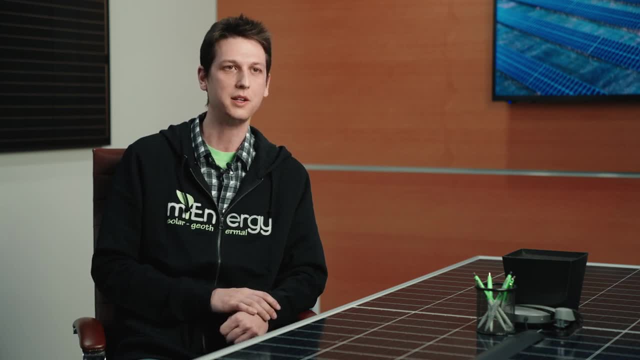 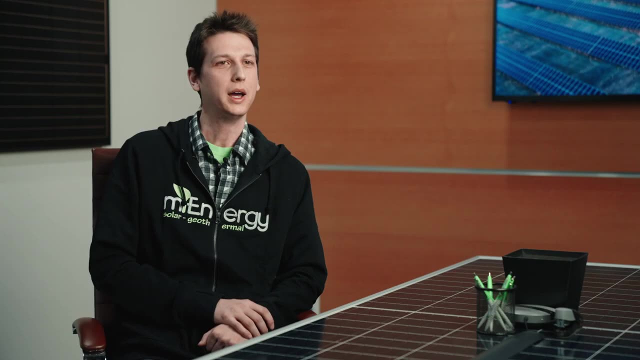 You're not watching the clock. It's always lots going on And it is satisfying when you know that you're making a difference and what you're doing is having a positive impact. So it was something where, when I got into it at the time, there was maybe only one or two companies in the problem. 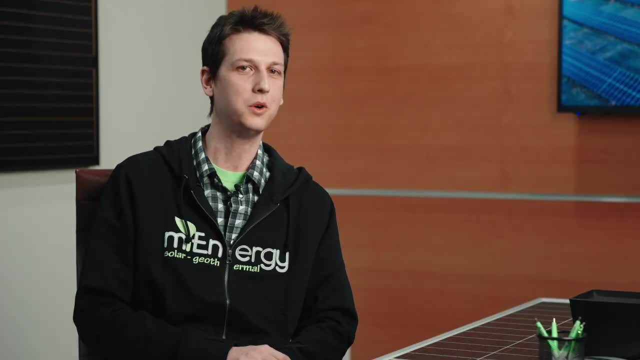 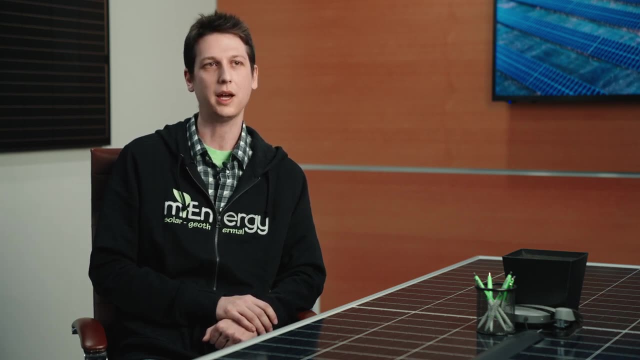 It's doing solar. So when I was searching around for jobs, it was one of those things was like I've never seen that before. I did the kind of few projects in school. It was something that always interested me And something that kind of resonates with me as a person is being an expert in what you're doing. 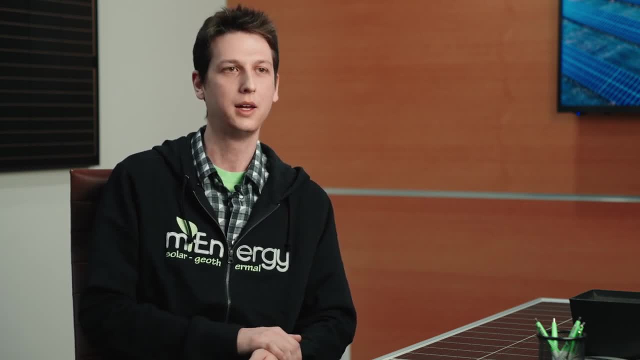 And I'd like that to be unique as well, And this was a perfect fit for that where it's like: this is a brand new industry, It's growing, It's in its infancy And I'm kind of getting in at the ground level. 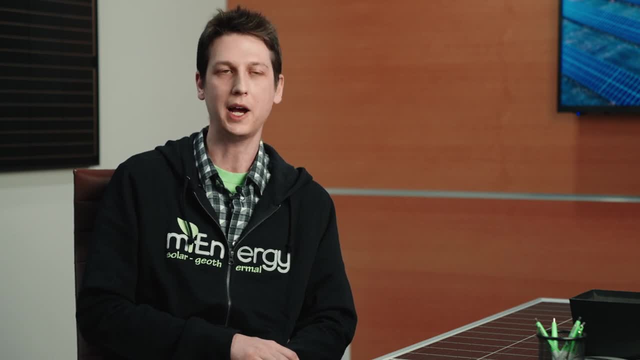 And that's kind of where I found that kind of attraction to the industry, Where it's like, hey, this is brand new and there is a huge ceiling. That's kind of what you always hear when you're in school or when you're a kid. 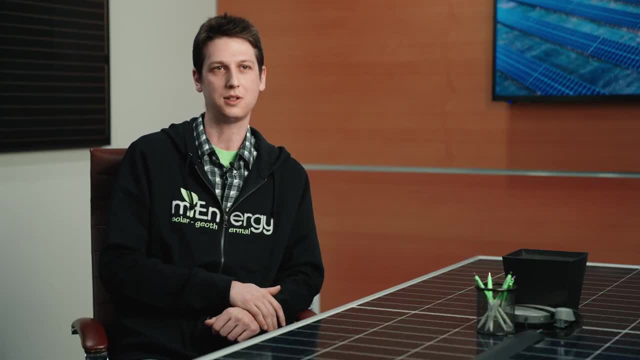 It's like if you can find something that has a lot of potential for growth or is a new and exploding industry, that could be very interesting for lots of kids- And that was for me too- where it's like, hey, there's so much room to grow here and actually be a part of something that your work is showing results. 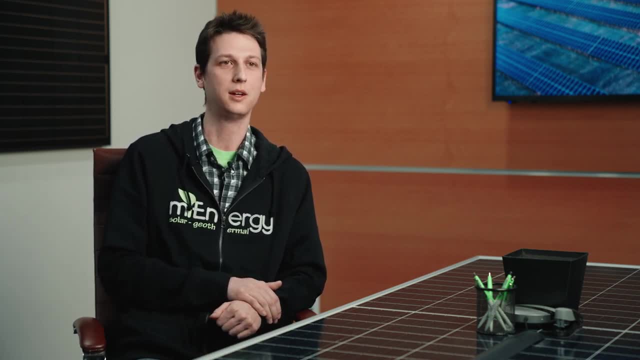 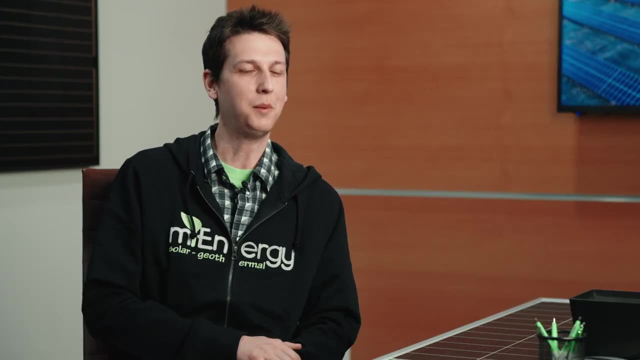 And you can see that like hard work is like, yeah, this is really something I've taken off and I've had a decent input into that, So that was something that I find very valuable. Probably the most enjoyable is seeing that impact. Your hard work getting in at the ground level and growing with a smaller company as it gets bigger and bigger with the industry has been really rewarding. Where I can see that I started on the tools on the roof and then kind of growing and growing and the company is growing and the industry is growing. 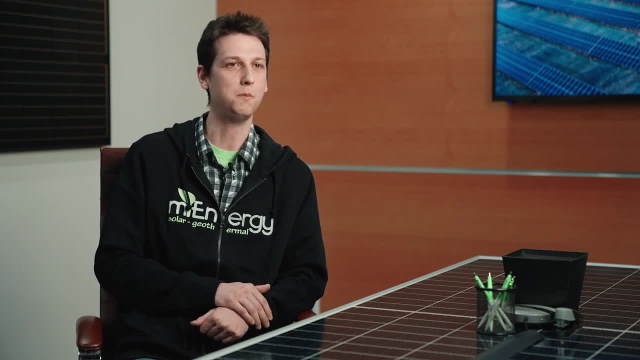 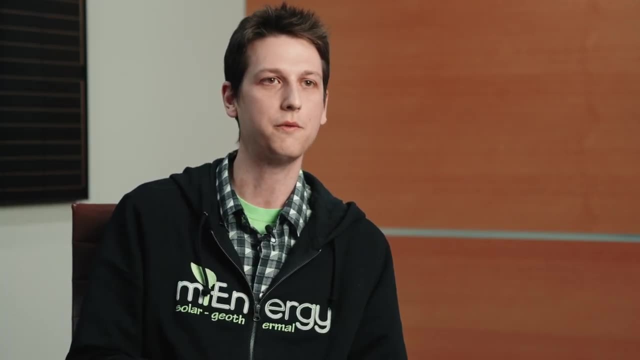 And you can see that it's like, hey, this feels really good And I like kind of being part of that progression where the industry is growing. I'm learning at the same time and growing and kind of feeling like, hey, this has all been a really good choice and it's been successful. 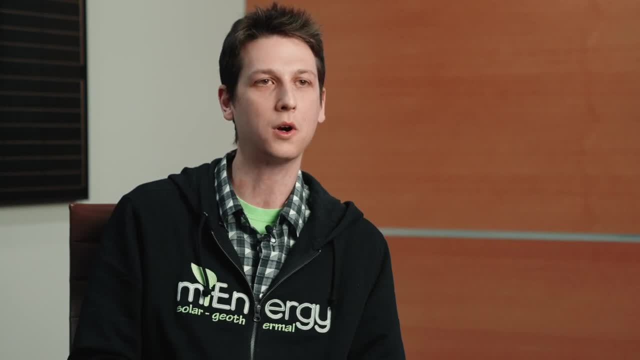 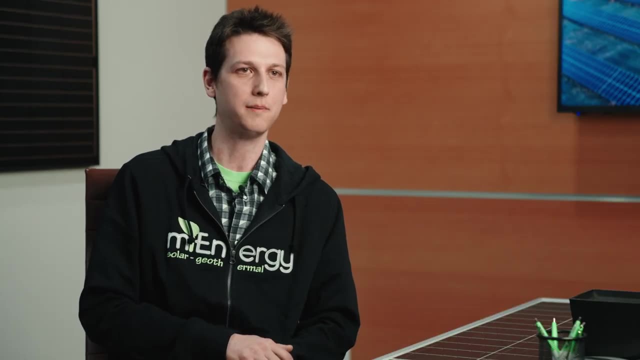 So that's kind of what I like it When I come to work. I know that this has been a good choice and it was smart to kind of pursue this career path. Yeah, here in Saskatchewan it's similar to pretty much most places in the world. 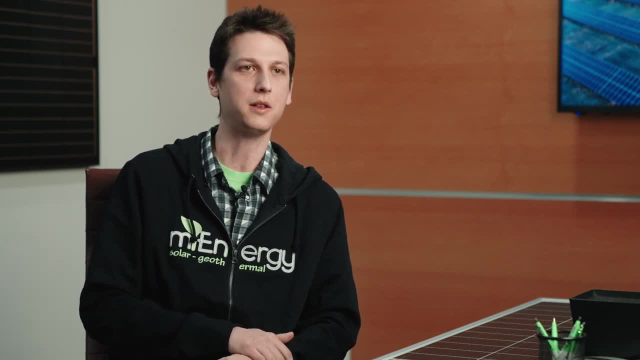 Solar is growing, Renewable energies are growing. The interest is there, right, The population and the people here Are interested in it, and it's the same way as everything, And in the past 10 years that I've been in the business it went, like I said, from one or two companies, a handful of people, to several different companies, big projects, lots happening and a lot of interest. 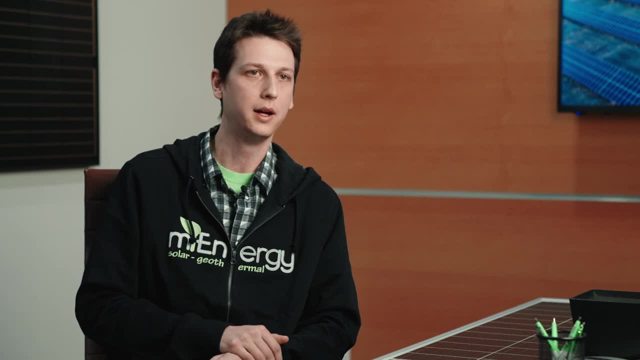 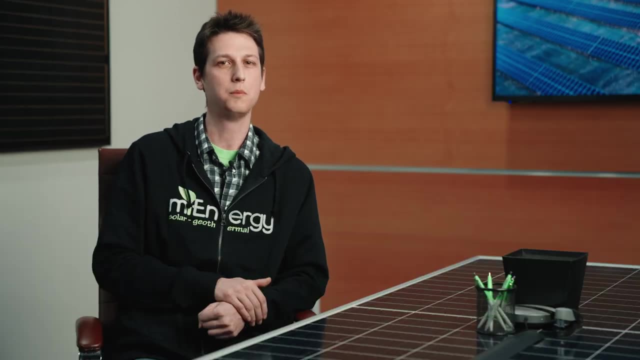 So I think the future is there for sure. It's not going anywhere. It keeps getting better And here in Saskatchewan, yeah, it's got a good future. We're seeing a lot of stuff happening and you might see on the news or on the Internet or wherever- big projects. 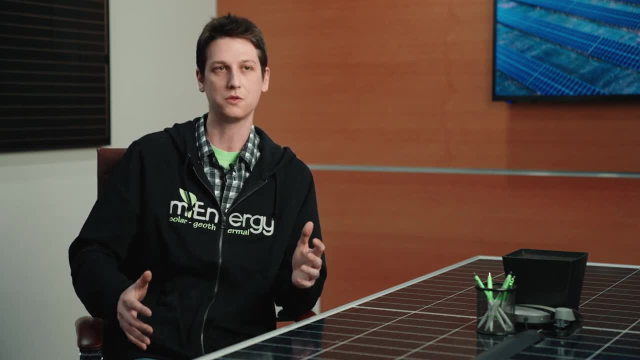 Well, those are happening here now. Those are starting. We're starting to see a big field of solar panels. I've been fortunate enough to work on a couple of those, So I think I think the future is really positive for science specifically. 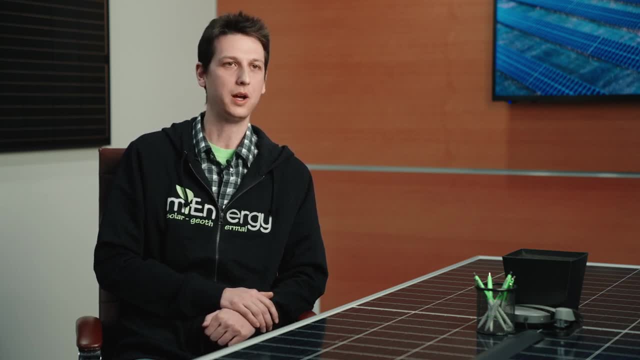 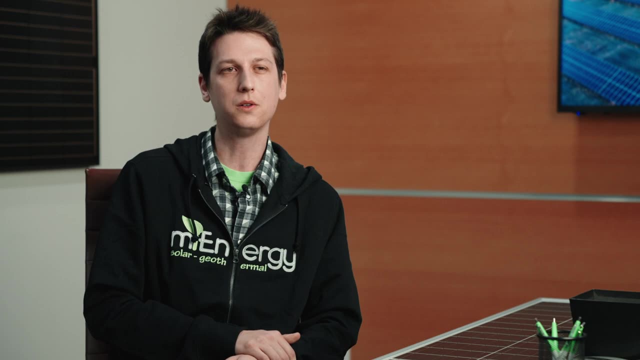 It's such a such a good field, It's so broad, right, You can do anything, You can go anywhere and fit in. So if you're, if you're thinking about sciences, whether it's renewables or anything, I think it's a fantastic field, or at least set of interests to pursue. 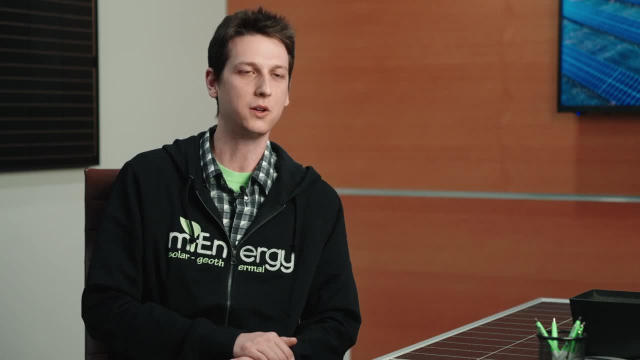 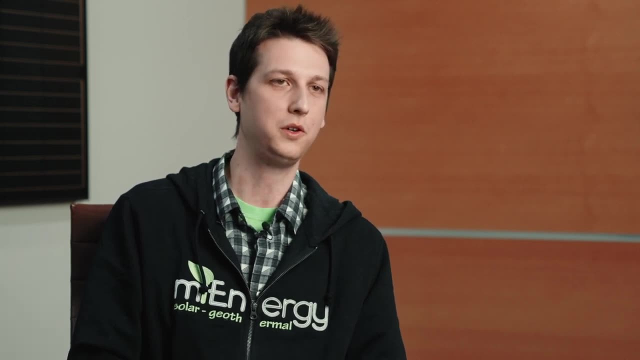 Like if it's something that interests you, you'll find something And I think you'll love it. Like if it's something that's your passion and you can, you'll find a career for it. if you're trying, If you're thinking about getting into renewables, the future is really positive. 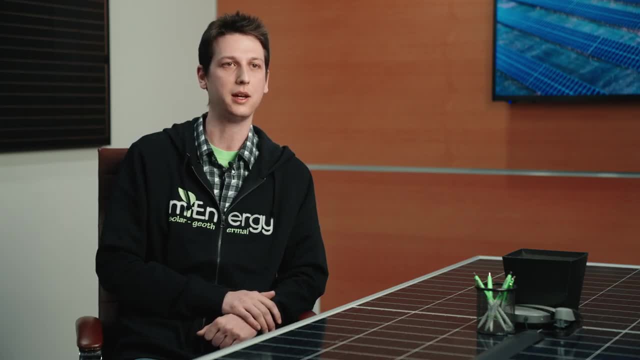 There's going to be a lot out there, lots of opportunities as the industries grow across Canada or even across the world. If you're looking at traveling or doing this elsewhere, there is a lot of potential. If traveling and being abroad isn't your thing, locally here in Saskatoon, there's a lot of. 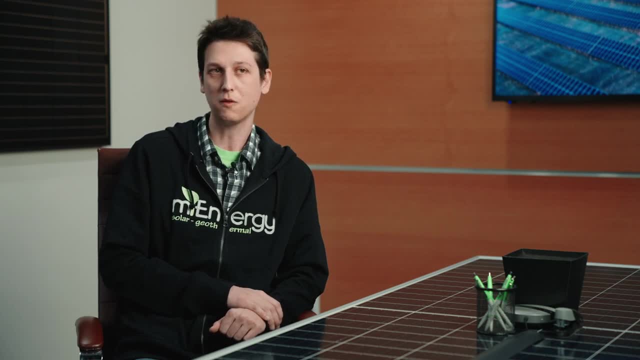 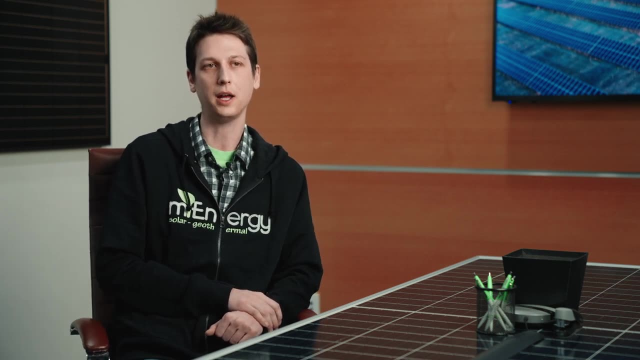 opportunity. The city is got a number of really good incentive programs that get homeowners and people thinking about: hey, it's easy to add solar now, So that's going to be a big and expanding market. The city of Saskatoon is also thinking about adding kind of what we call megawatt scale. 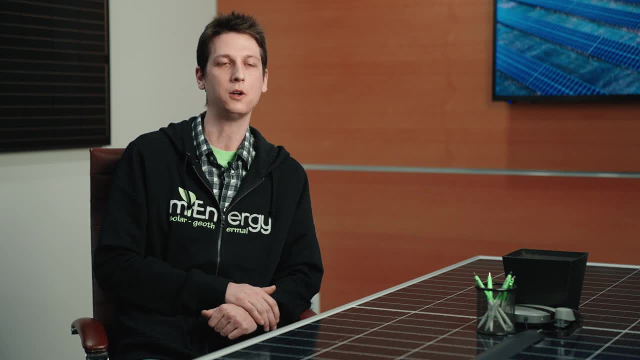 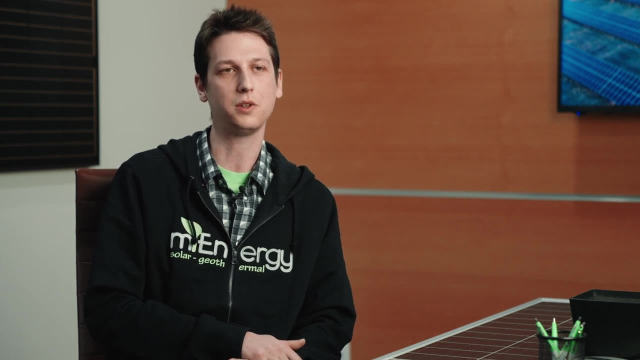 or a big solar field here in the city. There'll be that happening over the next few years where that'll bring a lot of attention and kind of show that hey, we're committed here in Saskatchewan, and specifically in Saskatoon, to doing solar and going green and doing renewable energy.